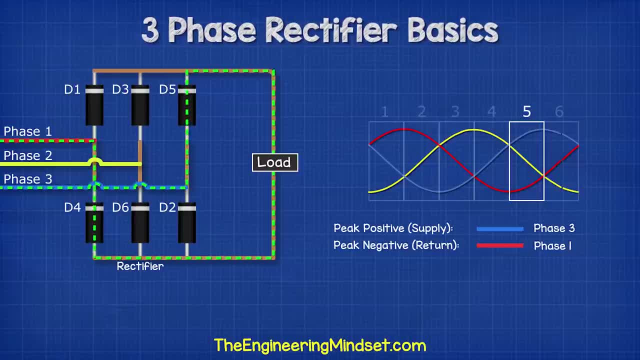 flows through this phase via diode five. It then flows through the load and then returns via diode phase 1.. Finally, the current flows through phase 3 via diode 5, through the load and then back into phase 2 via diode 6.. This cycle just repeats constantly, like this: 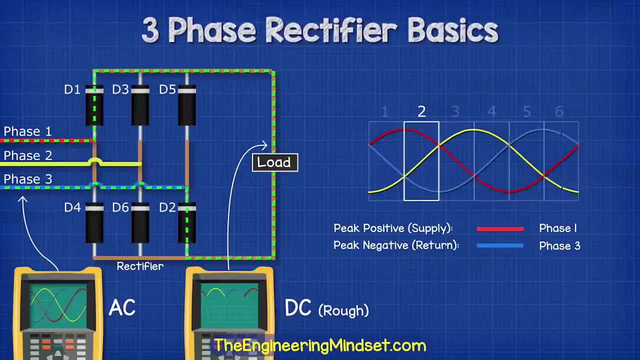 The oscilloscope for the 3 phase supply will see 3 sine waves for the AC electricity. But the oscilloscope on the load will see this as a rough DC electricity with some ripples in it. Now we need to smooth out those ripples to clean up the DC electricity. For this we 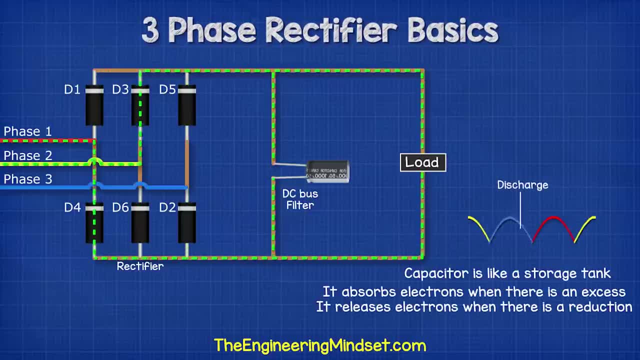 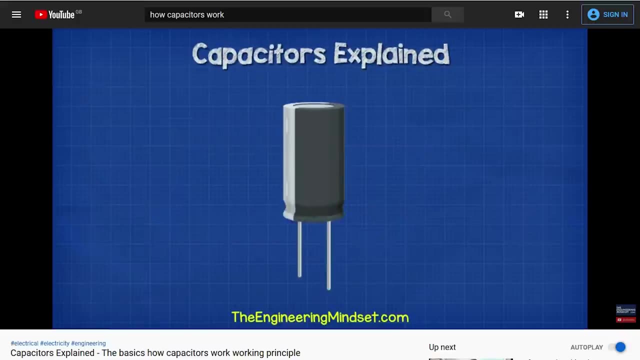 connect a capacitor across the positive and negative. This capacitor is like a storage tank and will absorb electrons when there is excess and it will inject electrons when there is a reduction. This will therefore smooth out the ripples in the DC electricity to a nice, smooth signal on the oscilloscope. We have covered capacitors in great detail. 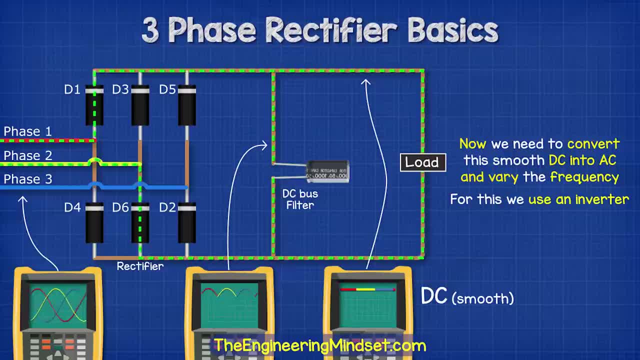 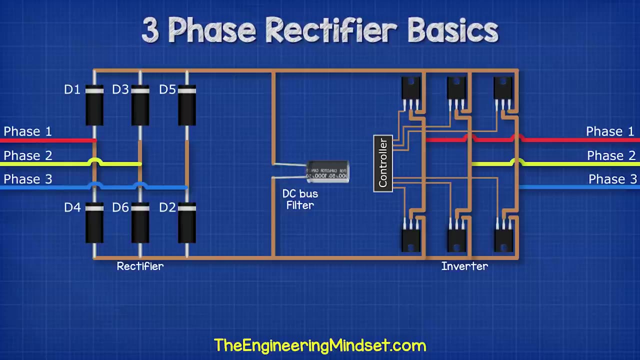 previously. Do check that video out. links down below. Now that we have clean DC, we're ready to turn that back into precisely controlled AC at variable frequency, and for that we need an inverter. An inverter is basically a number of IGBTs, which are switches that can turn on and off super fast. I'm going 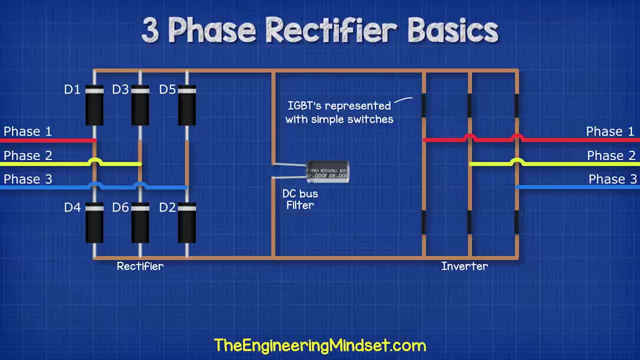 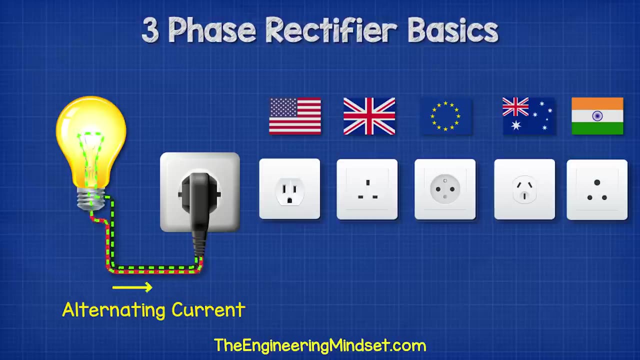 to animate this using some simple switches instead of IGBTs. just to make it easier to visualize, I'll number these switches as follows: To get our three phases we need to open and close switches in pairs to direct the flow of current from our supply and a return pass. That way the connected motor will. 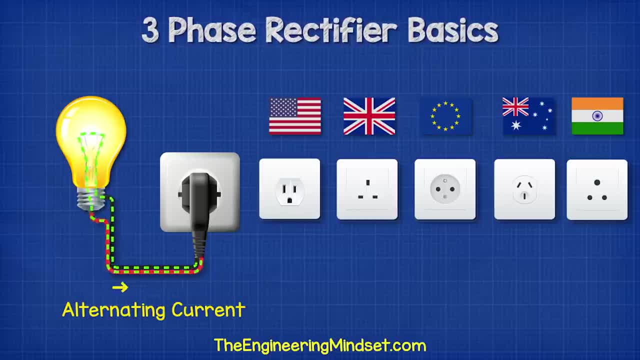 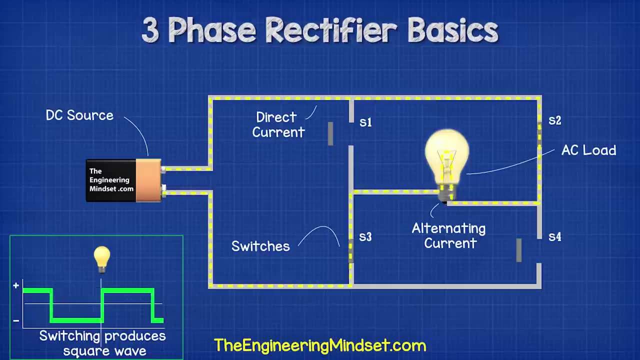 experience alternating current. Remember, AC is where the current reverses. So if we took a lamp and connected it to some switches and a DC power source, we can control the direction of current through the lamp by opening and closing switches in the right order. Therefore the lamp experiences alternating current even 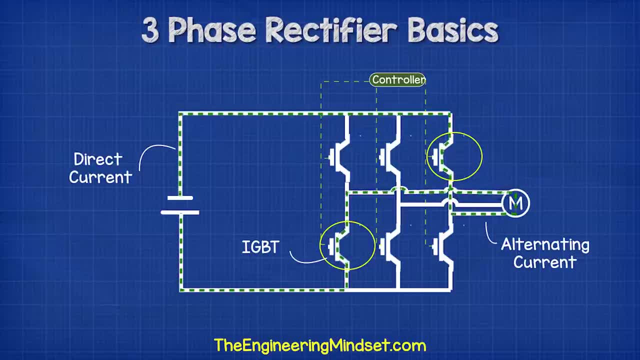 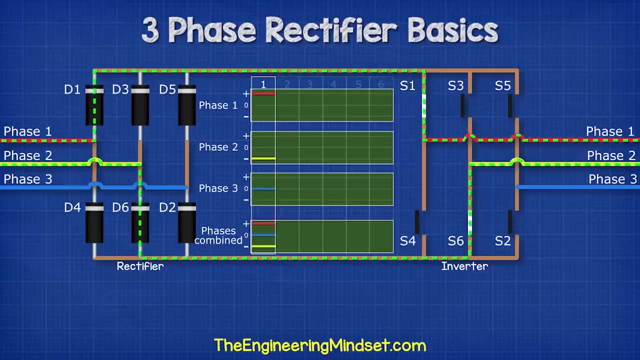 though it's coming from a DC supply. For the three-phase supply, we time the switches to simulate the three phases. Let's see how this works. First of all, we close switches one and six. This will give us phase one to phase two. Then we close switches one and two. This will give 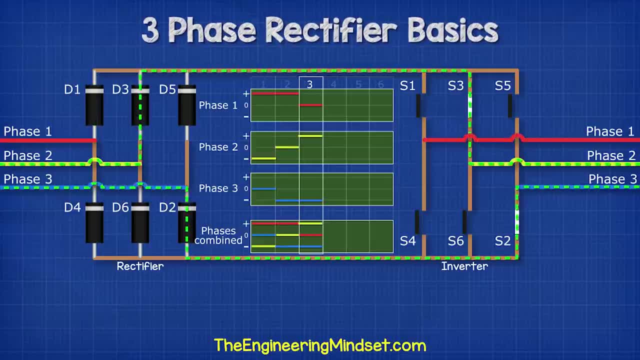 us phase one to phase three. Then we close switches three and two. This will give us phase two and phase three. Then we close switches three and four. That will give us phase two and one. Then we close switches five and four and this. 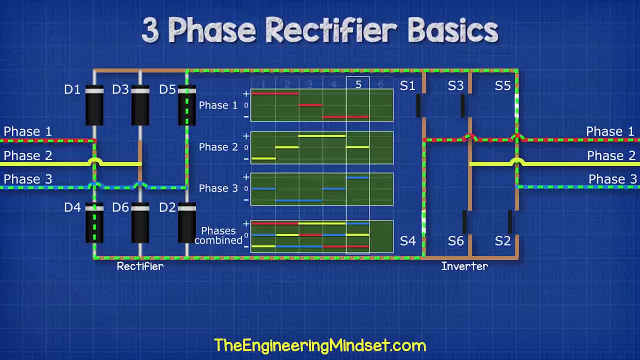 will give us phase three and phase four. Then we close switches three and four. That will give us phase two and one. Then we close switches five and four, and this will give us phase three and phase one. And finally we close switches five and six, and this will give us phase three and phase two. 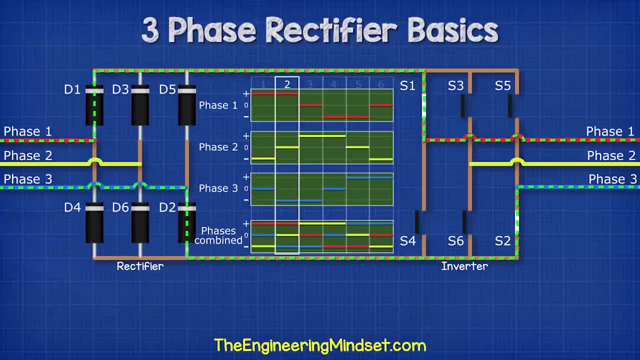 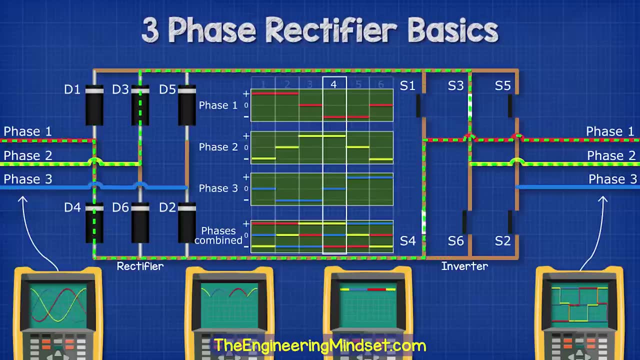 This cycle repeats again and again like so: If we check this with the oscilloscope, we now have a pattern that looks like a C sine wave, although it's just a little bit square. This will work fine for some applications, but not all. 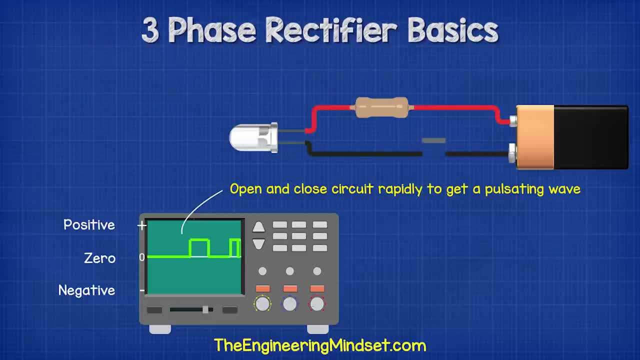 so how can we improve this? Do you remember? earlier in the video I said we can open and close the switch at different speeds and durations to change the waveform. Well, we can do that with this too. What we do is use a controller to rapidly open and close the switches multiple. 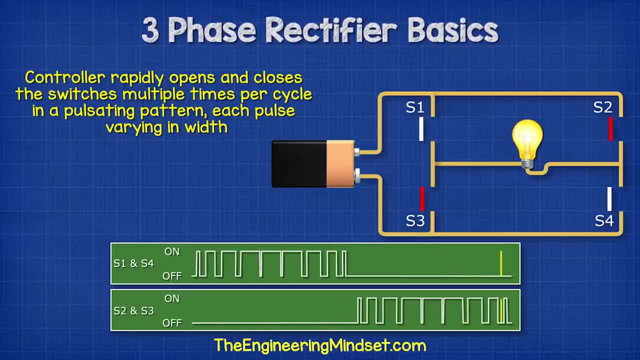 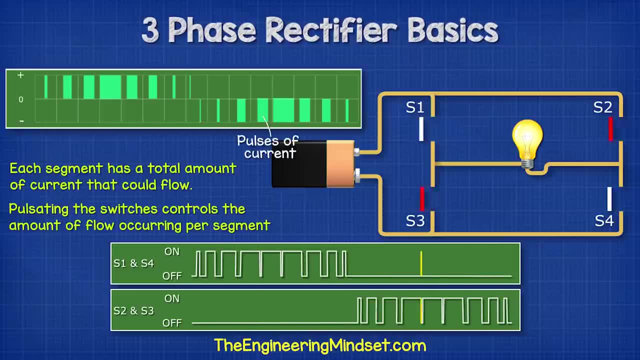 times per cycle in a pulsating pattern, each pulse varying in width. This is known as pulse width modulation. The cycle is broken up into multiple smaller segments. Each segment has a total amount of current that could flow, But by rapidly pulsating the switches, we control the 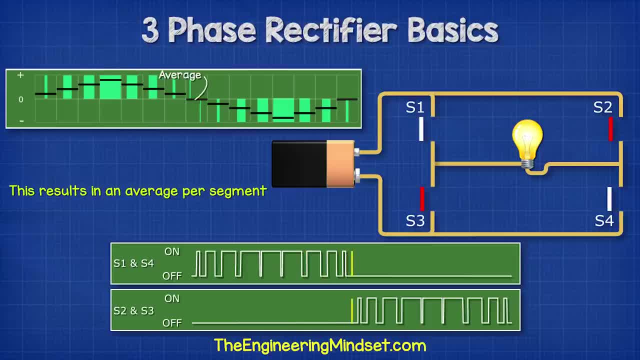 amount of current that could flow, But by rapidly pulsating the switches, we control the amount of flow occurring per segment. This will result in an average current per segment and we can see that this increases and decreases, thus giving us a wave pattern. The load therefore experiences a sine wave. 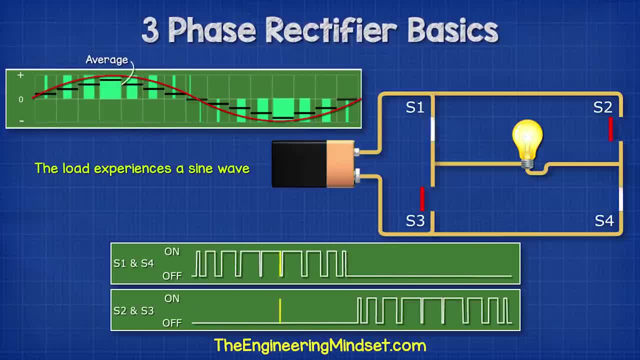 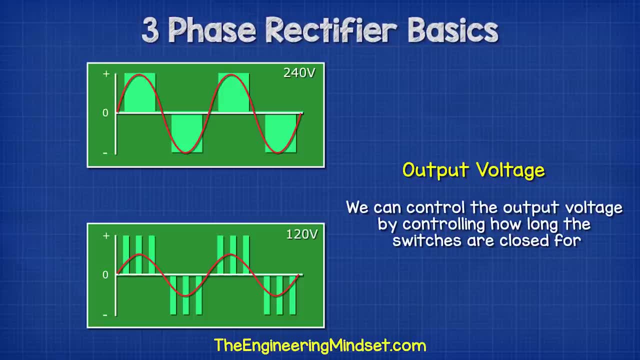 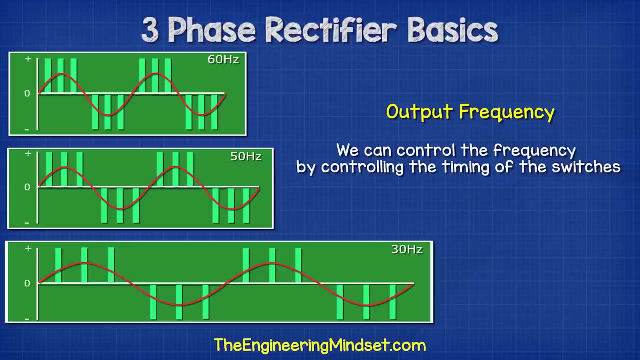 The more segments we have, the closer it will mimic a sine wave. We can control the output voltage by controlling how long the switches are closed for. So we could, for example, output 240 volts or 120 volts just by trimming the opening and closing times. We can control the frequency by controlling the timing of the switches. 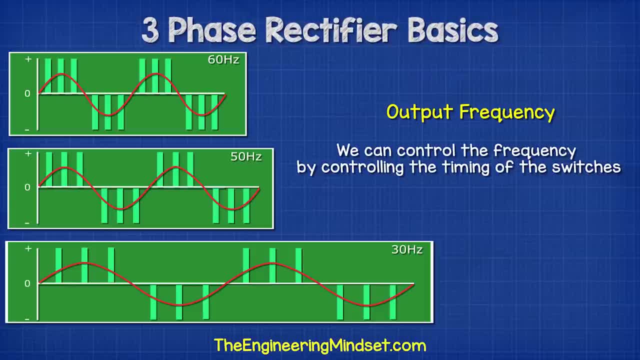 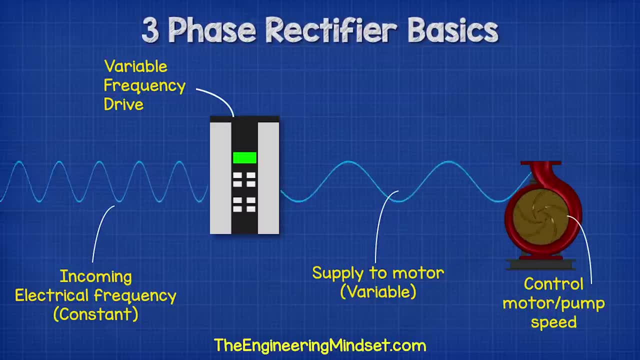 So we could, for example, output 60 hertz, 50 hertz or 30 hertz, whatever is needed for the application. Remember, by controlling the frequency we control the rotational speed of the motor. So, coming back to our VFD circuit, we're going to use the controller to rapidly open and close the